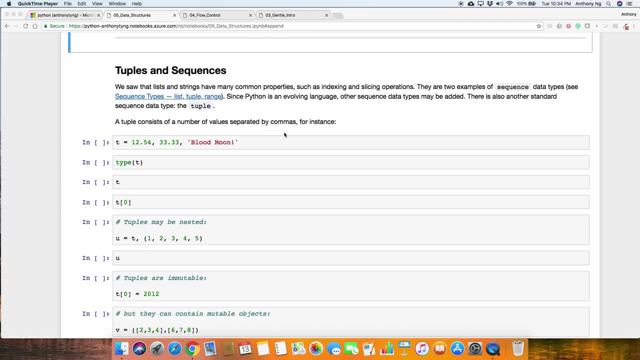 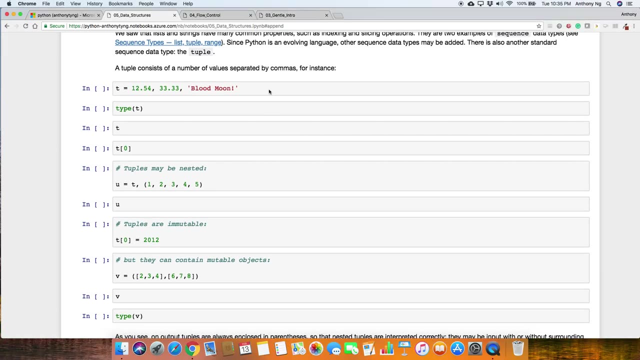 link, if you like. Now, Python is an evolving language. Other sequence data types may be added in the future. There's also another standard sequence data types which is called tuple. Now, tuple consists of a number of values separated by a comma. Now the example of this. 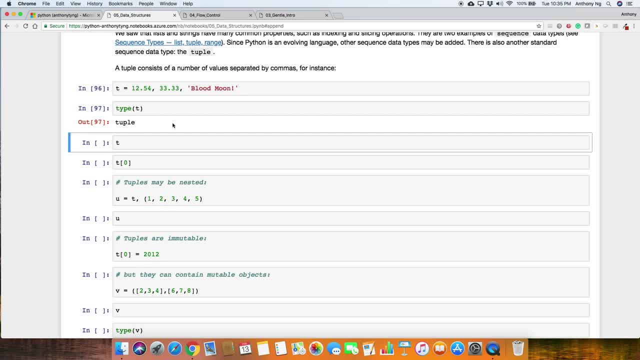 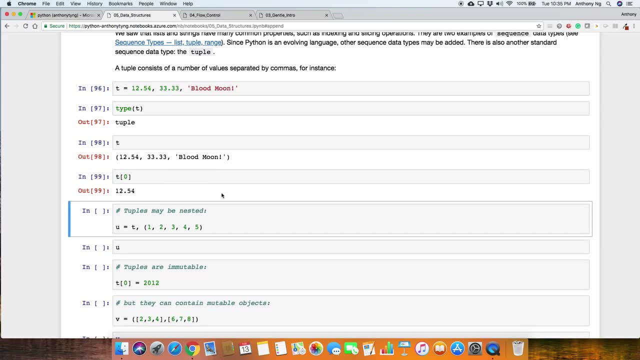 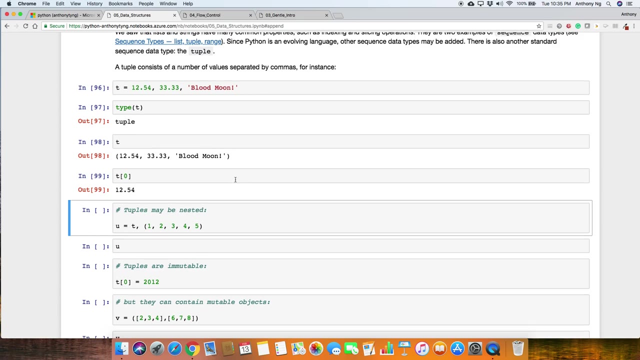 remember we use type bracket, whatever the variable is, to check what it is. So here you have. this is actually a tuple. Now again you can actually do indexing. That gives you 12.5.. Notice that tuple has a bracket to it. Tuples may be nested as well. That's what now you have. 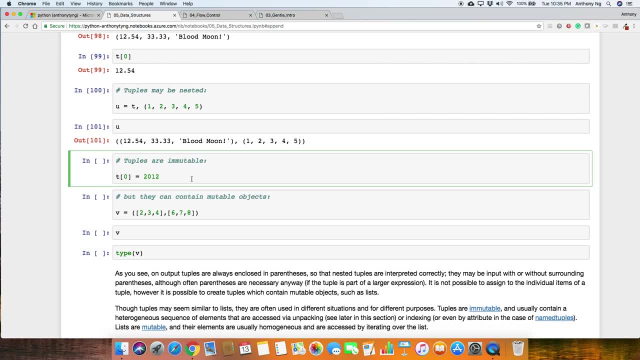 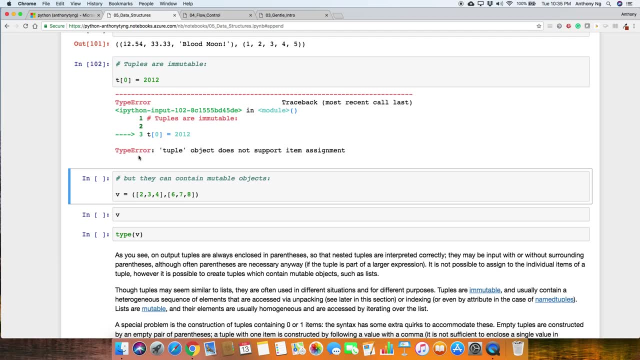 u, as the actual tuple Tuples are actually immutable, So that means you cannot change the value, much like string. Hence you actually have a type error here. It does not support items assignment, But they can contain mutable objects. Okay, so v. here is actually a list. 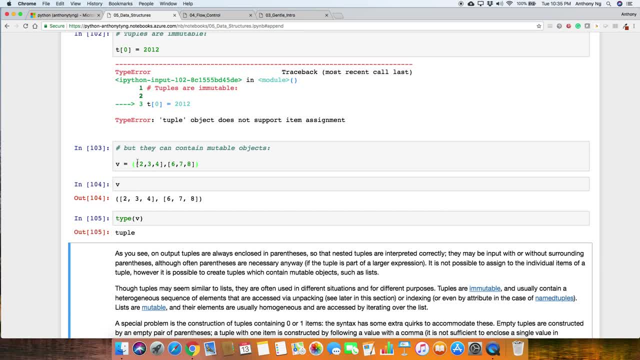 And notice that v is not a list, sorry. Inside here is actually a list. 2,, 3,, 4 is a list, 6,, 7,, 8 is a list, But the bracket means that the v is actually a tuple From what you can. 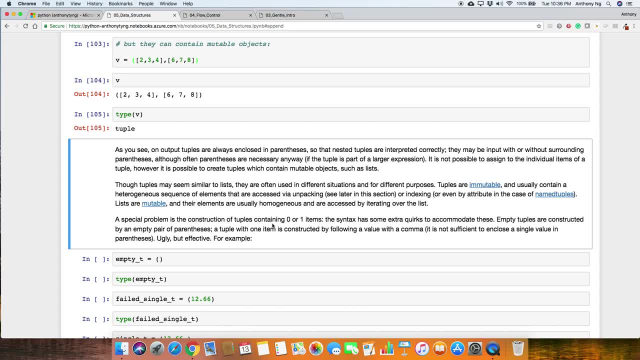 see here is that an output tuple are always enclosed in parenthesis So that nested tuples are interpreted correctly. They may be input with or without surrounding parenthesis, although often parenthesis are necessary. Anyway, it is not possible to assign to the individual items of a tuple. However it is. 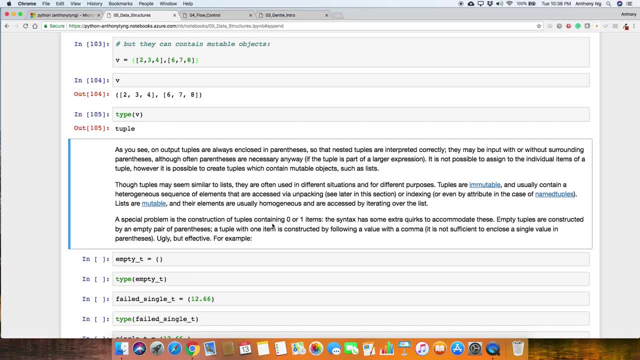 possible to create a tuple which contain mutable objects such as list, which is what we did here. We created a tuple with mutable objects which are list. Now, tuple may look similar to list. They're often used in different situations and for different purposes. Tuples are immutables and usually contain heterogeneous sequence. 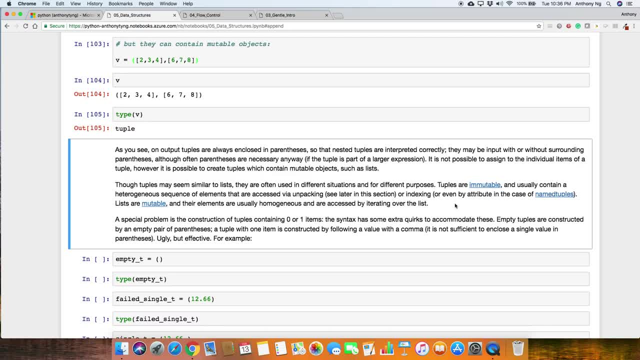 of elements. They are accessed via unpacking or indexing. Lists are mutable and their elements are usually homogeneous and are accessed by iterating over the list. Notice, therein lies the actual key difference. Tuples are typically because it's immutable, they are accessed via and they are often. 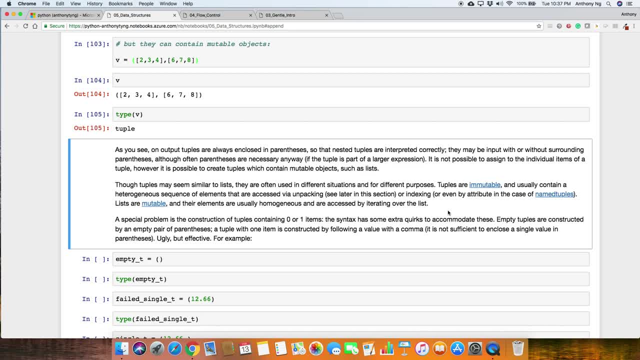 heterogeneous, meaning they have different types of data types, and usually you access it by unpacking or indexing. That's one. Lists are mutable. They are accessed via a single point. They are usually accessed via an iterative type of data type, So you are actually able to do a lot of things with a tuple. 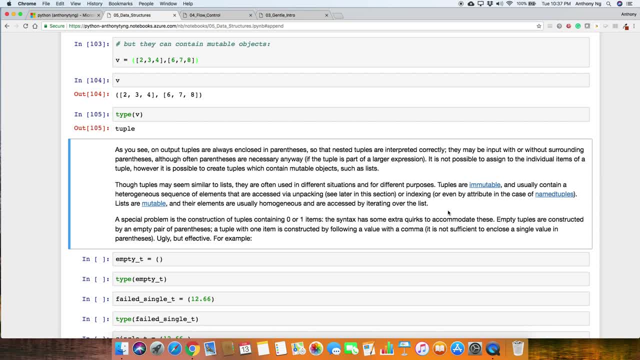 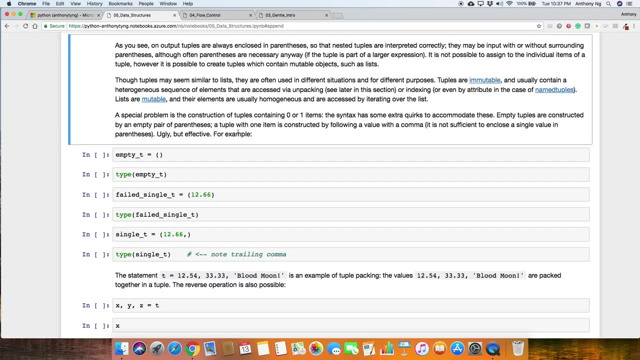 A special problem is the construction of tuples containing 0 or 1 item. The syntax has some extra quirks. Empty tuples are constructed by an empty pair of parenthesis. A tuple of one item is constructed by following a value with a comma. It is not sufficient to enclose a single value in parentheses. 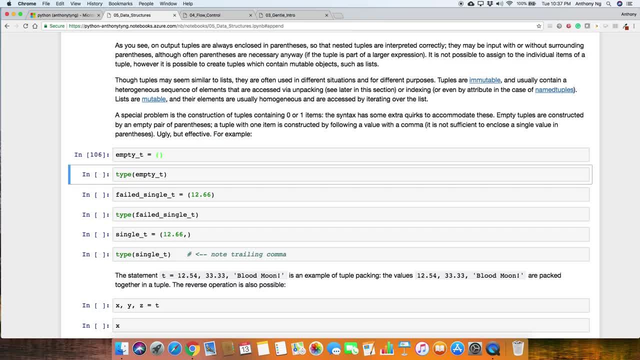 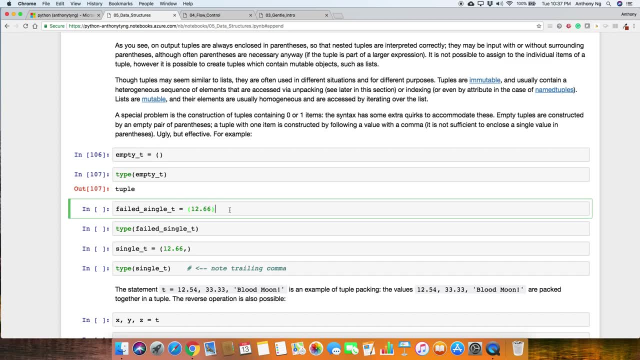 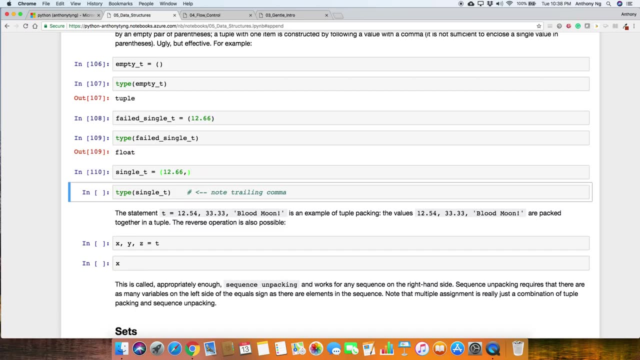 Ugly but effective. So if you're creating an empty tuple tuple, you just use the bracket, so that's fine. But if you try to do this, this is not a tuple. okay, It's just not a tuple. But if you put a comma, it's fine. Okay, so it's. 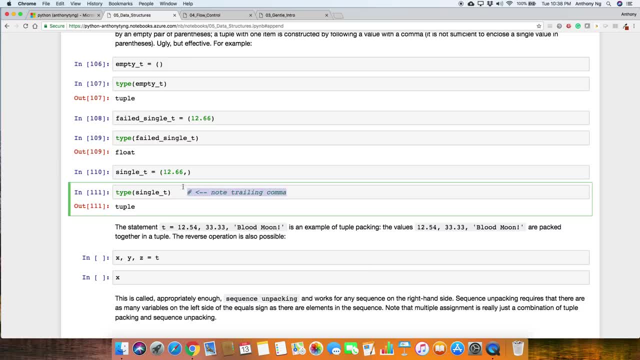 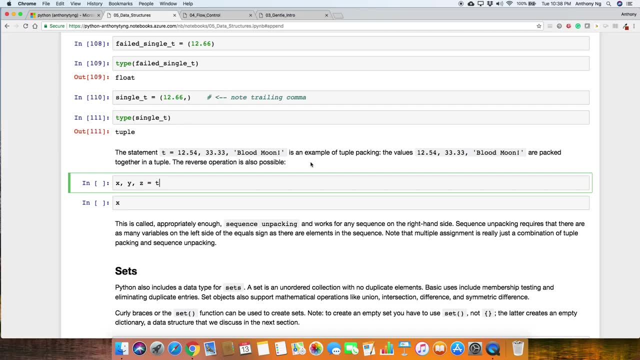 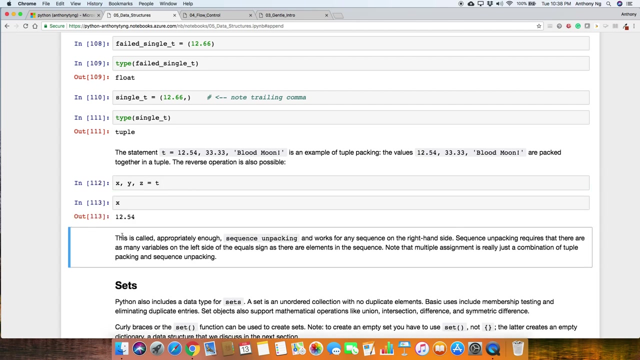 perfectly fine, So this should actually technically be over here: 1,, 2,, 3, 4.. Okay, the statement: this is an example of tuple packing The values. these are packed together in a tuple. The reverse equation or operation is possible. Basically, you have x, y, z unpacking it and you have 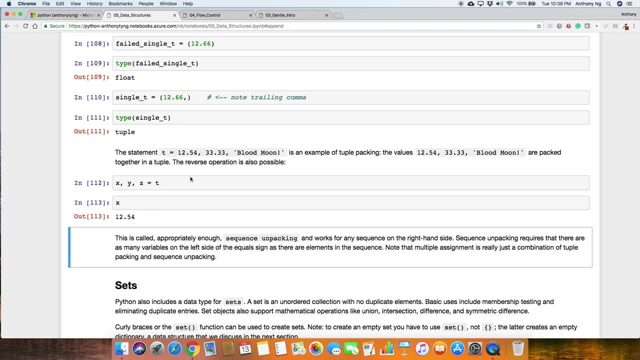 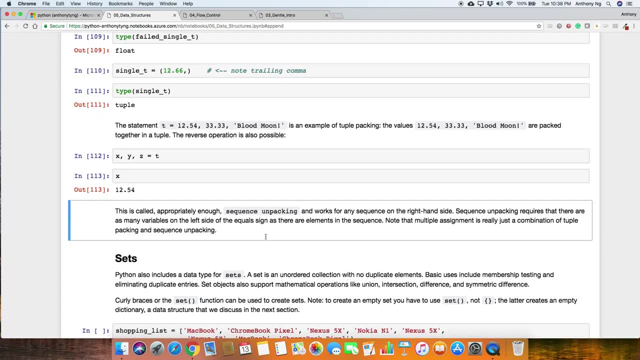 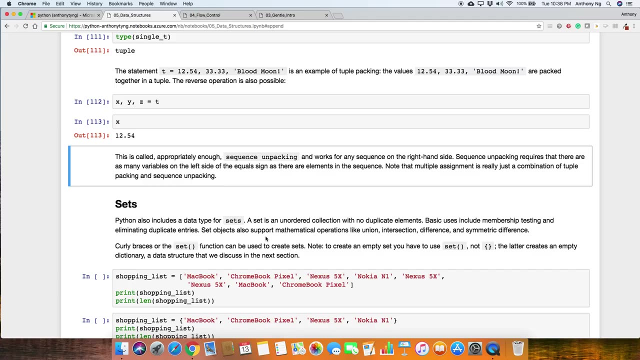 the first stored to x. second value stored to z. the last value stored to z. Okay, so this has become x, this becomes y, this becomes z. by unpacking it this way, This is called, appropriately enough, sequence unpacking. It works for any sequence on the right-hand side. Sequence unpacking requires that there. 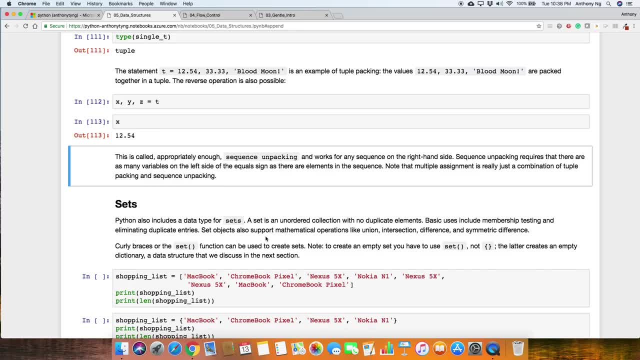 are as many variables on the left side of the equal signs as there are elements on the sequence. So that means the number of variables on the left must equal to the number of elements, otherwise you're going to get an error. Okay, note that multiple assignment is really just. 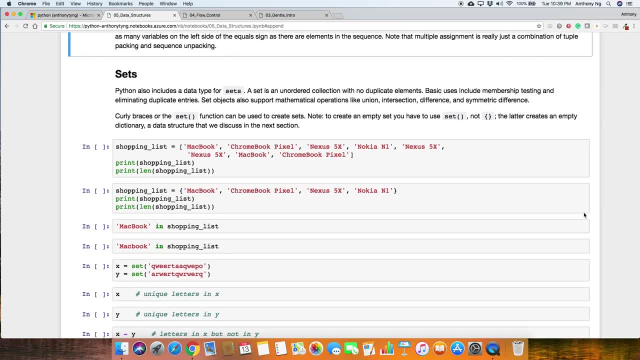 a combination of tuple packing and sequence unpacking. Right. so with that, I'm going to stop. In the next video. we're going to go into sets.